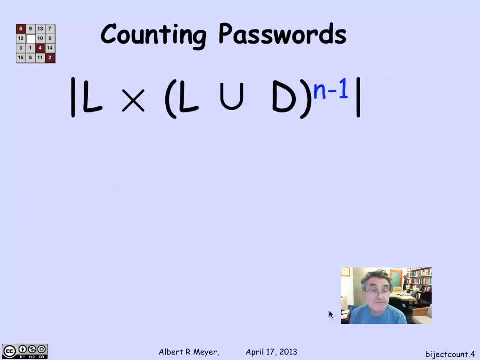 D cross L union D cross L union D N minus one times. Well, now we have an easy way to count this, because the size of this nth power is going This product by the product rule, is the size of L times the size of L union D. 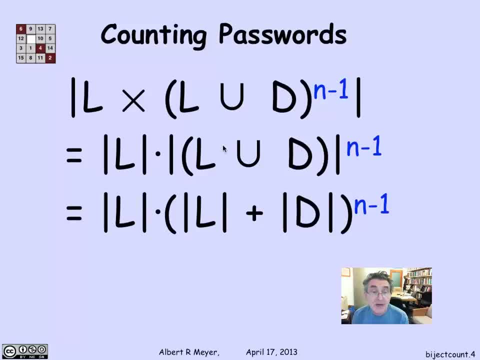 to the n minus first power And of course L union D. since letters and digits don't overlap, by the sum rule, the size of them is just L plus D, And so I get this nice formula that it's 52 letters times 52 letters plus 10 digits raised. 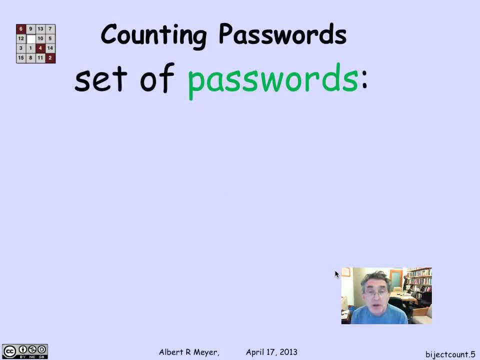 to the n minus first power. OK, what about the passwords? Well, the passwords were then P6, union, P7, union, P8.. And since words of length 6 don't overlap with words of length 7 or 8, this is a disjoint union. 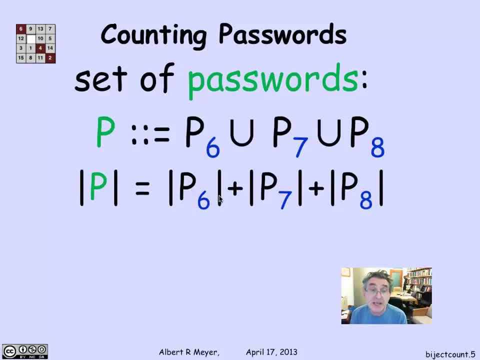 And therefore the total number of passwords as specified is simply the size of P6 plus the size of P7 plus the size of P8.. There's the formula. when I plug in And it turns out to be a good size number: 19 times 10. 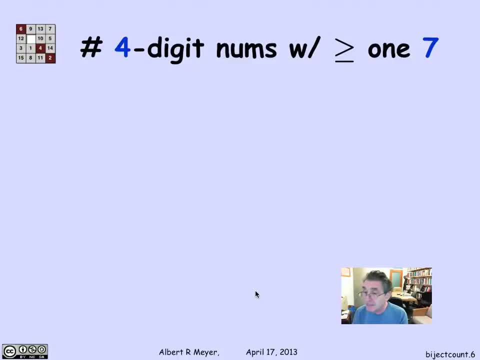 to the 14th- OK, that's one simple example where I'm translating a spec- And to something that I can express easily as a products and disjoint sums of stuff that I already know the size of. Let's just do another example. 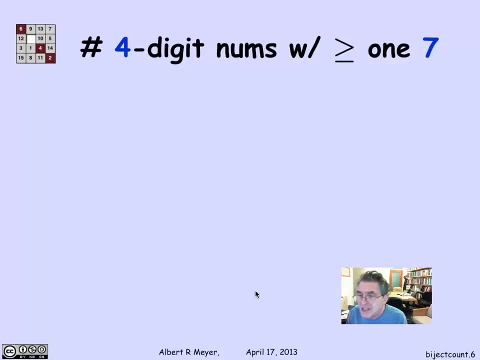 Suppose that I want to count the number of four-digit numbers. So the elements of these four-digit numbers are 0 through 9.. There are 10 possibilities With at least one 7, the number of four-digit sequences of digits And the number of numbers that have at least one 7 in them. 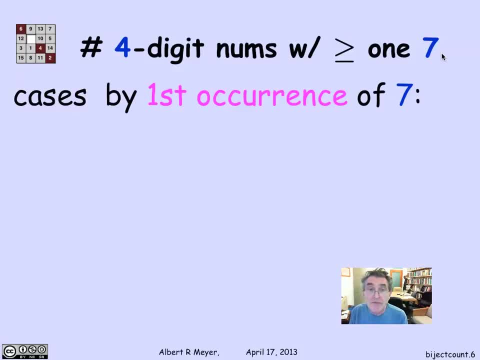 And one way to count is: I can make it a sum of different four-digit numbers containing one 7, depending on where the first 7 is. If there's at least one 7, there's a first 7.. That's the well-ordering principle being applied. 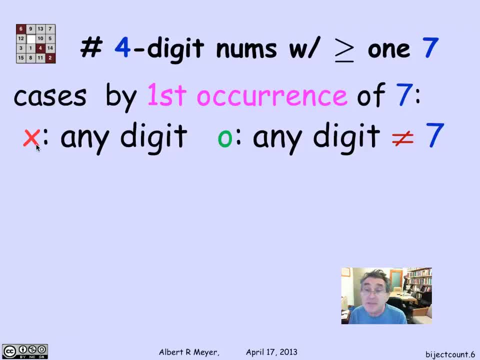 So if we let x abbreviate any digit, there are 10 possible values of x, and o represent any digit other than 7, so there's nine possible values of o. then the words that start with 7 can then be followed with any three digits. 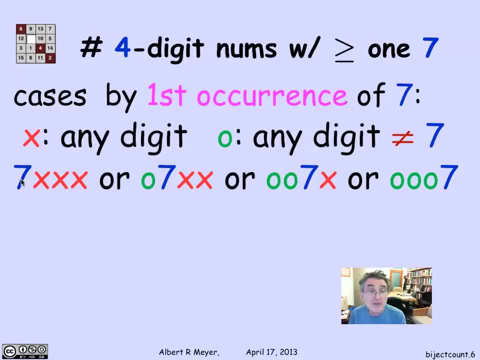 So 7xxx is one possible pattern when the first occurrence of 7 is first. Another possible pattern is when you have a digit that's not 7, followed by a 7. This is when 7 occurs second, followed by anything at all. 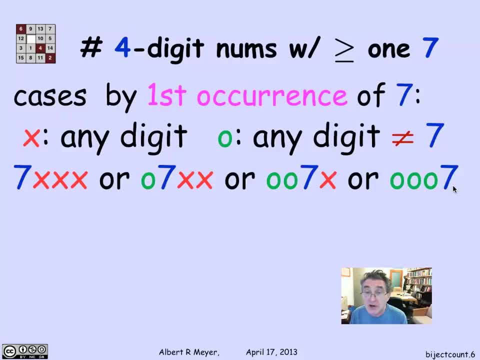 Likewise, here 7 occurs third and here 7 occurs fourth. Now these individual patterns are easy enough to count using the product rule, Because if you have a number that's not 7, then you can't count it. Here I have to count how many triples of any digits are there. 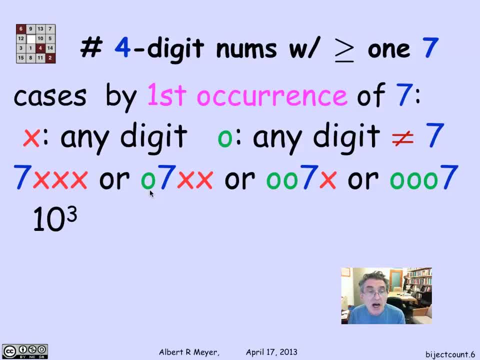 Well, there's 10 digits, so it's 10 cubed. Here. how many sequences of where the first choice is 9, and the second two choices are the 10, and it's 9 times 10 squared. Here it's 9 squared times 10, and here it's 9 cubed. 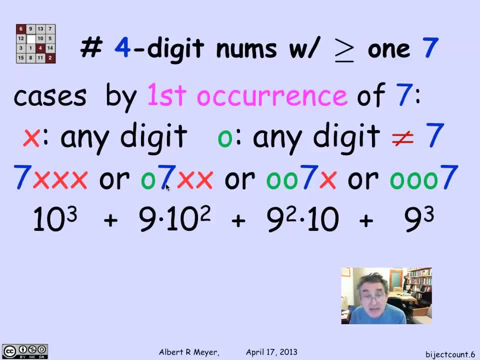 These are disjoint because they're distinguished by where the first 7 occurs, And so I just add them up and I get this number and it's not especially interesting, but it's 3439.. OK, So that's an exercise in counting something. 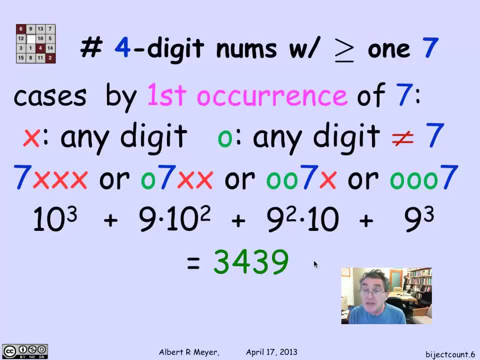 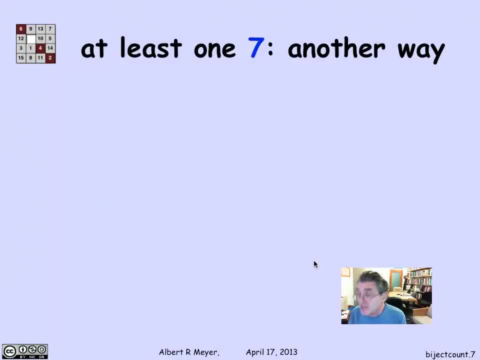 by somewhat ingeniously breaking it up into a sum of disjoint things that are themselves easier to count. There's another way. that's another standard trick that comes up in combinatorics of how do you count the sequence of four-digit numbers with at least one: 7,. 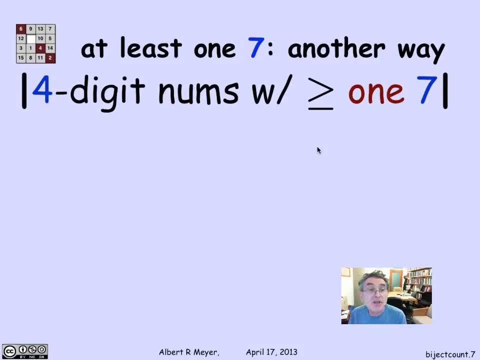 by counting their complement. Count the numbers of four-digit numbers that don't have any 7s and simply subtract that number- the number of four-digit numbers with no 7s- from the total number of four-digit numbers, and that's going to be the numbers that are left over. that 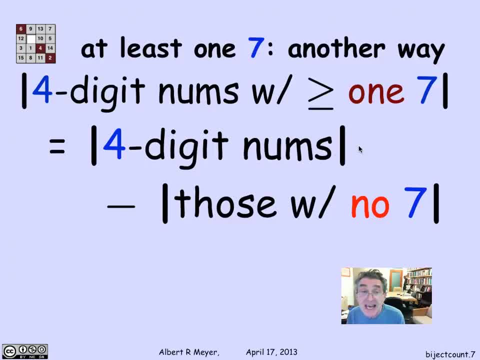 have one, 7.. Now the number of four-digit numbers is easy to count, and it will turn out that the number of four-digit numbers with no 7s is also really easy to count, because the number of four-digit numbers is 10 to the fourth. 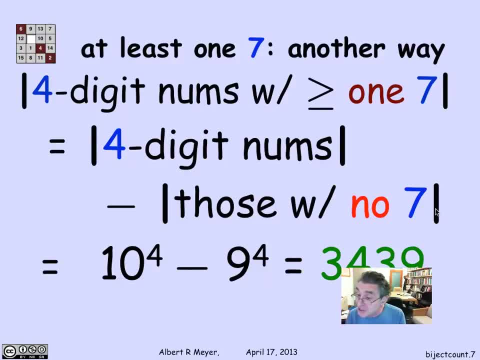 and the number of four-digit numbers. with no 7s, there's nine possible choices for each of the remaining digits, So it's just the digits 0 through 9, leaving out 7, to the fourth power or 9 to the fourth. 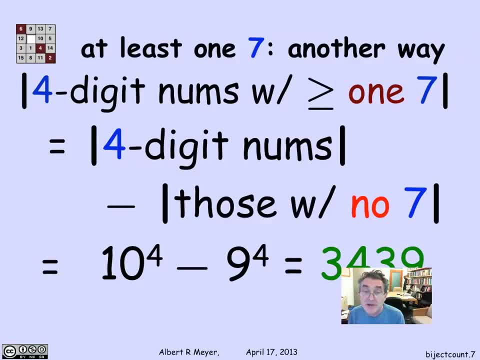 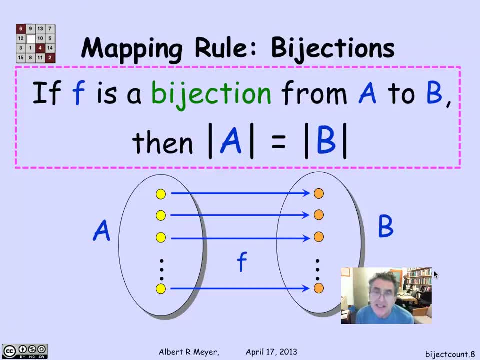 And you can double check that: 10 to the fourth minus 9 to the fourth is 3439.. So now, with that practice, using the basic sum and product rules, we can start applying and thinking about the bijection rules. So the bijection rule simply says: 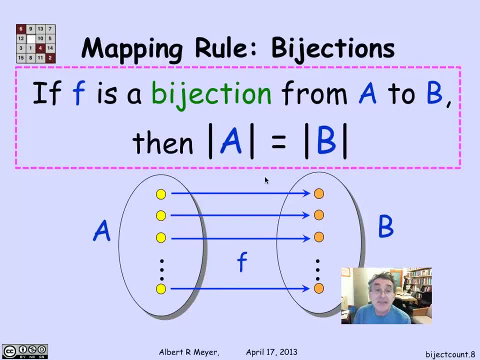 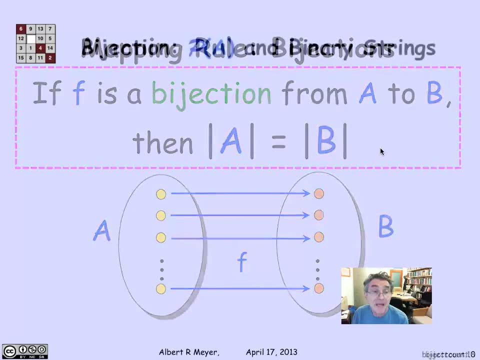 that if I have a bijection between two sets, A and B, then they have the same size, at least assuming that they're finite sets and the only kind of things we're counting are finite sets. Let's use an example of that where 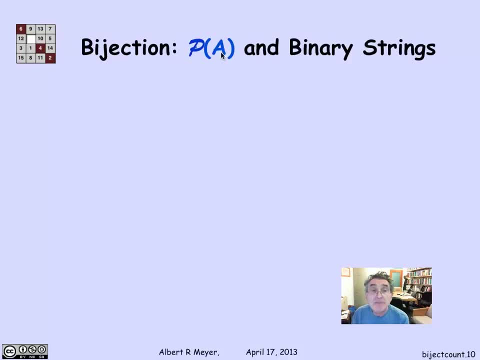 I'm going to count the number of subsets of a set A by finding a bijection between the subsets of a set A and something that I do know how to count. In fact, we've already counted them: The binary strings of a given length. 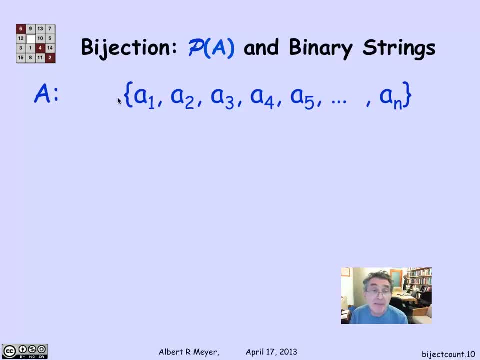 What's the bijection? Well, suppose that A is a set of n elements, Call them A1 through An, And I have some arbitrary subset of A. Say it's got A1, and it doesn't have A2, and it has A3, and it has A4,. 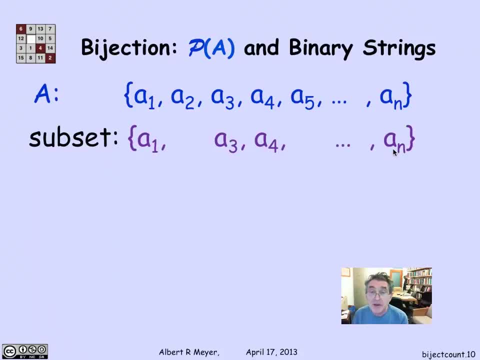 and it doesn't have A5, and then it's got some selection of the other numbers and it turns out it has An in it. Well, if I think of a subset laid out this way up against the corresponding elements in A, I can code this in an obvious way. 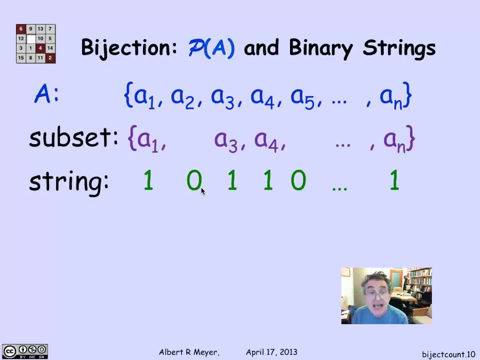 by putting a 1 where the element is in the subset and a 0 where the element is not in the subset. In effect, this is the so-called characteristic function of the subset, where 1 means that that index element, a 1 in the ith position, means that Ai is there. 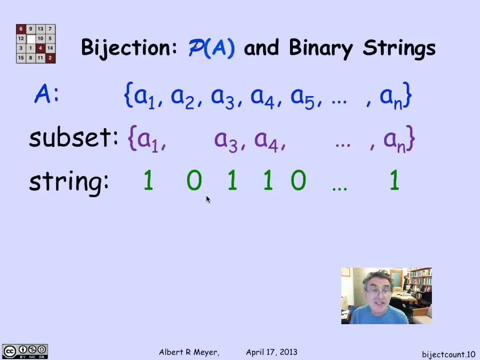 and a 0 in the ith position means that Ai is not there. So the second coordinate here is a 0.. That means A2 is not there And this is easily seen to be a bijection. That is, given the string, you can figure out. 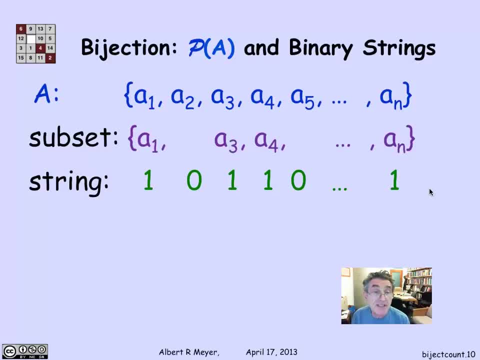 what the subset is. Given the subset, you can figure out what the unique string is. So we have a bijection, And what we conclude then is that the number of n-bit strings is equal to the size of power set of A. It's equal to the number of subsets of A. 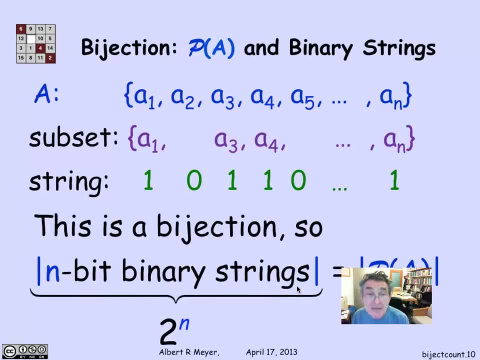 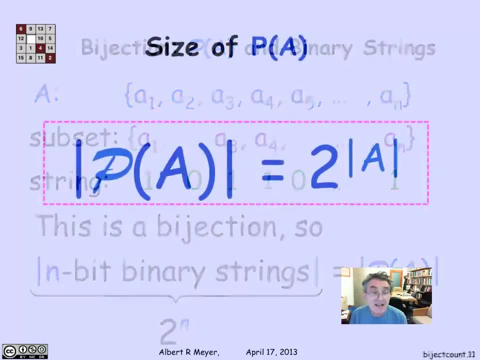 And of course we know how to count the number of n-bit strings: It's 2 to the n. So what we just figured out is: if I have a set of size n, it's got 2 to the n subsets. And a slick way to say that without mentioning n. 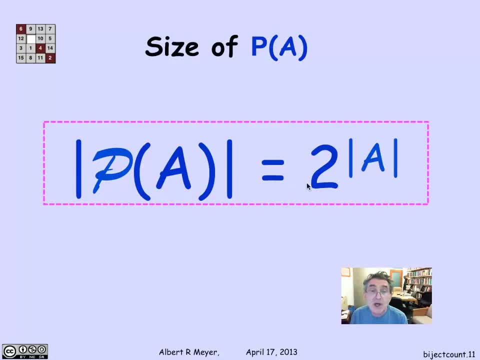 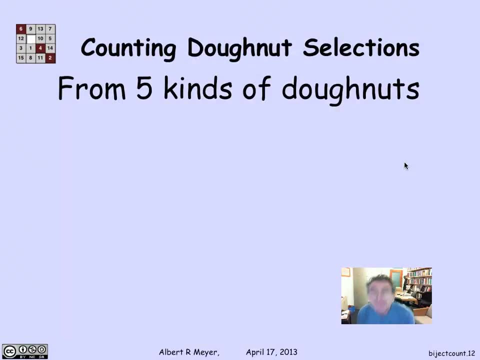 is that the size of the power set of A is simply 2 to the size of A. One more example of bijection counting. that is kind of fun and interesting and will illustrate the fact that we learn something by finding a bijection, even if we don't know. 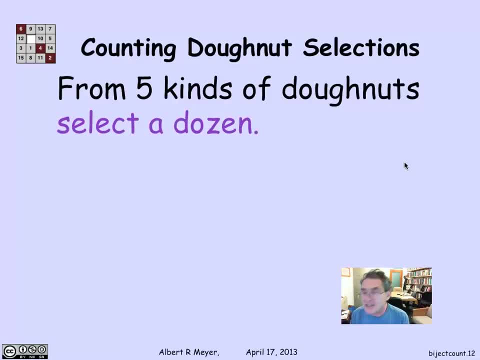 how to count either one yet. So what I'm interested in is: suppose I have a situation where there are five kinds of donuts, five different flavors of donuts, And I want to sort of select a dozen. I want to know how many selections there are. 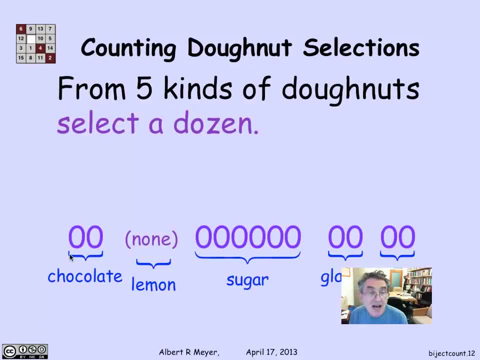 So, for example, these little o's represent donuts. I might choose a selection of a dozen by choosing two chocolate and no lemon- I don't like those so much- And six sugars, and two glazed and two plain. So there are 12 donuts here using four out of the five. 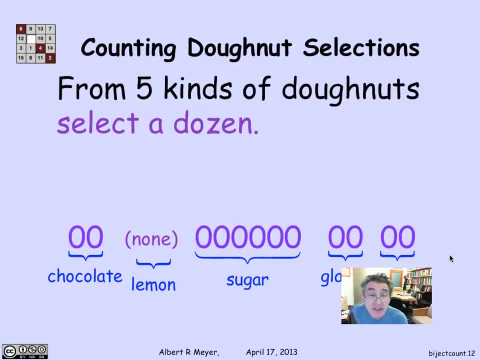 possible flavors of donuts. This is what I'll call a selection of a donut, and I'd like to know how many such selections of donuts are there. Well, let that be the set A, the set of all these different ways of selecting 12 donuts. 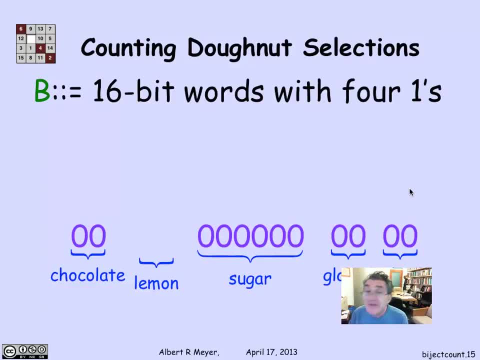 when there are five flavors of donuts available. Well, there's again an obvious correspondence between the set A of donut selections and the set B of zeros and ones of length 16 that contain four ones. What's the correspondence? Well, here's my donut selection. 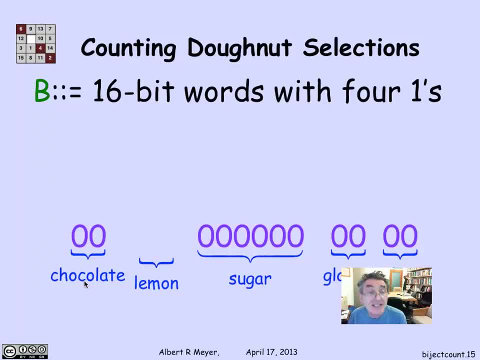 And of course the reason why I use those o's for donuts is that they also correspond to zeros. I can just put in ones as delimiters between the groups of flavors. So after the chocolate donuts I put a one, And then after the lemon donuts that happen to be none. 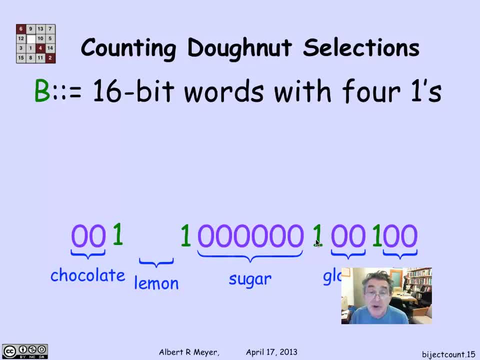 I put another one, And then, after the six sugar donuts, I put a one, And then I kind of consolidate and I extract from the donut selection this 16-bit word with one, 12 zeros, corresponding to 12 donuts and four ones. 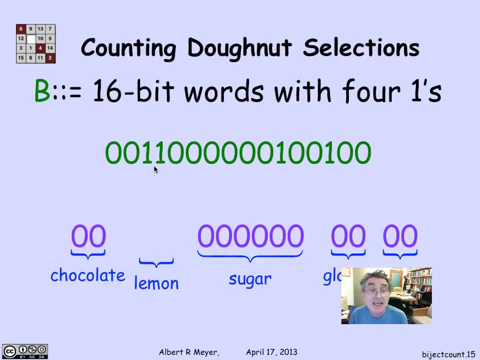 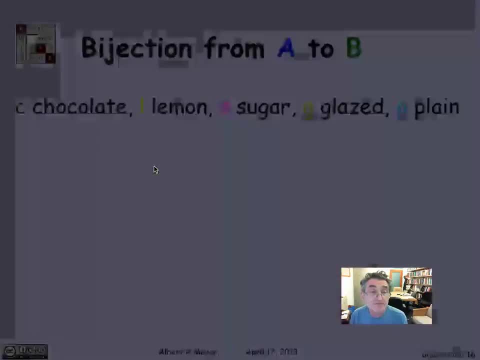 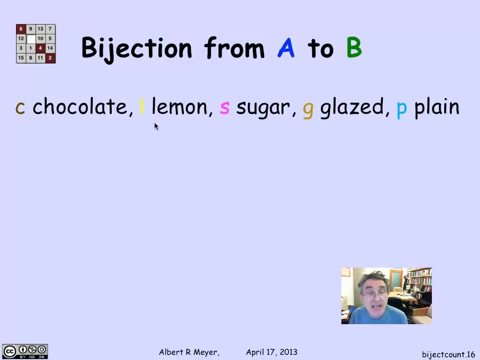 corresponding to breaking up those groups of zeros into five categories, five slots corresponding to the number of donuts of each flavor. So the general bijection, of course, is that if I have a selection of C, chocolate donuts, L, lemon,